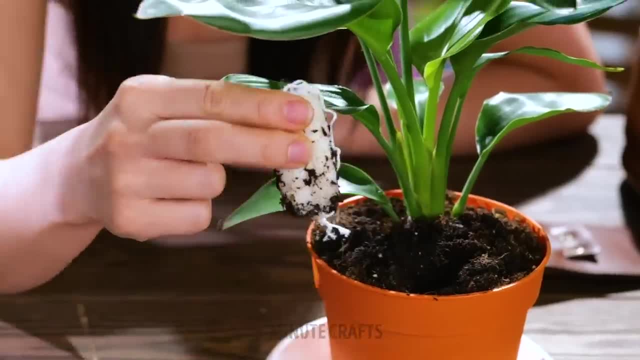 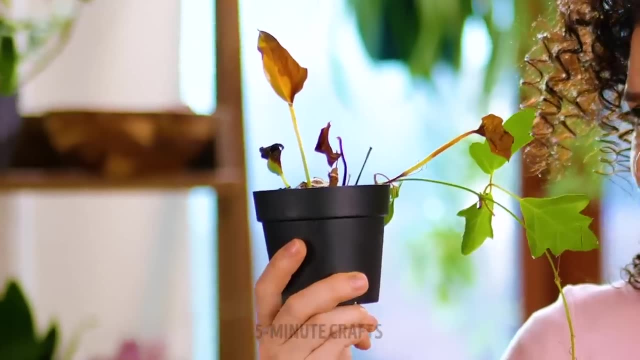 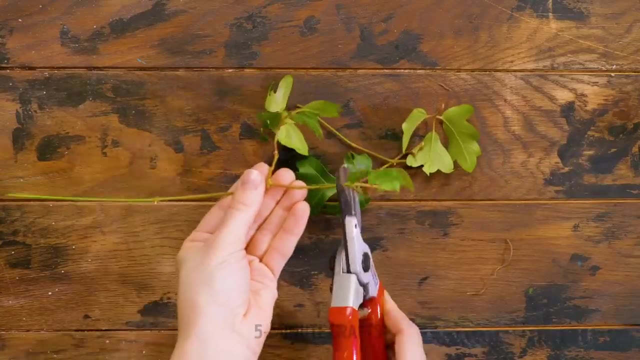 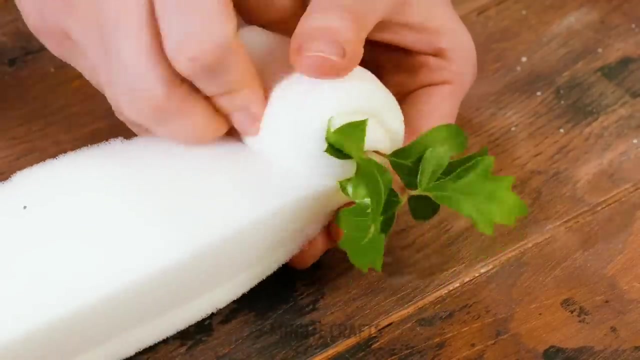 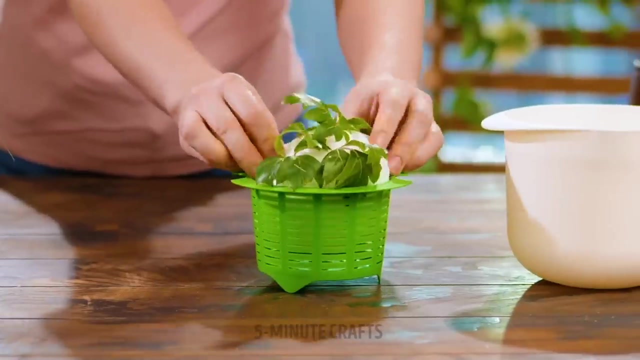 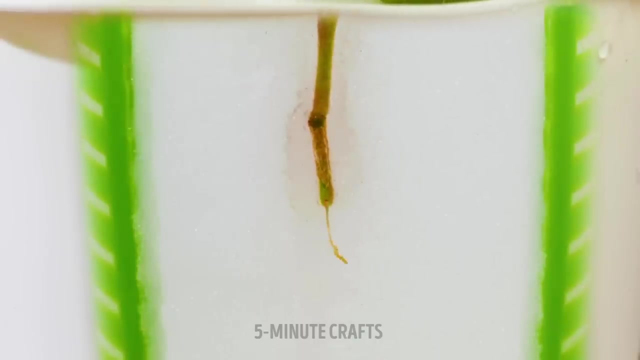 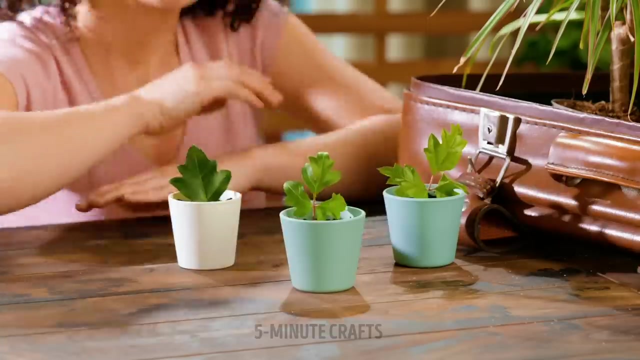 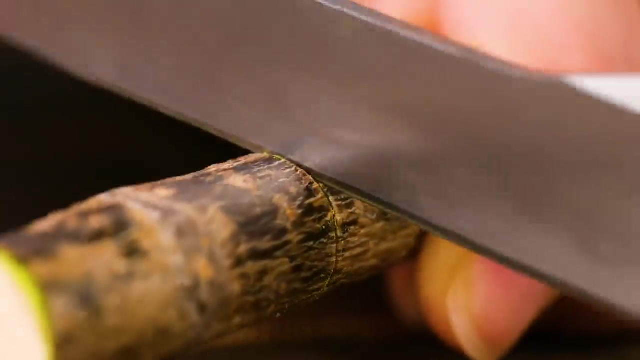 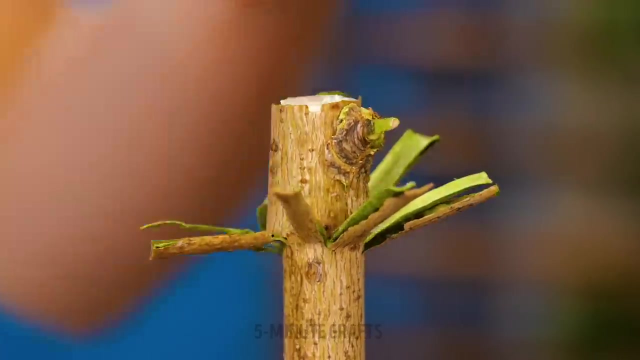 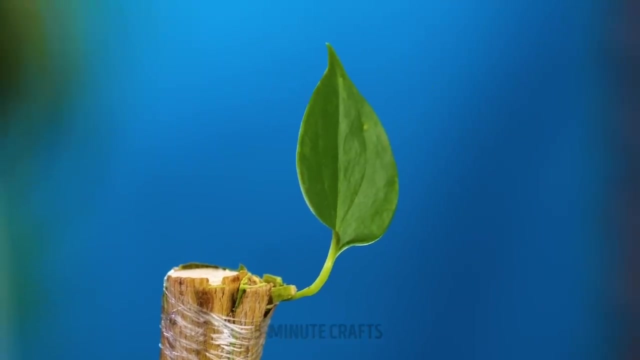 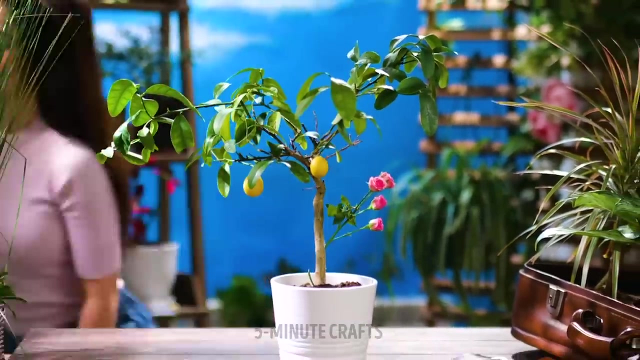 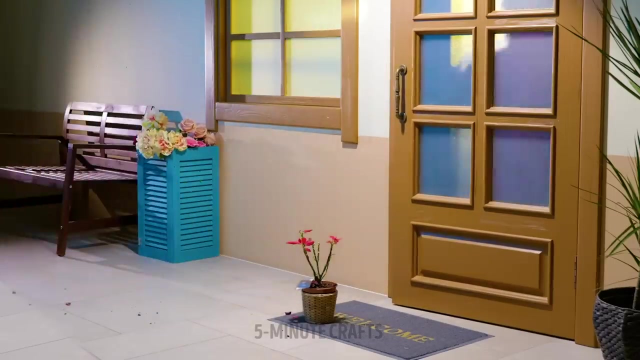 We'll be right back. We'll be right back. Yeah, I know it's in my head, Still I can't remember what you said. I know we've been here once before, The same old story. we just can't ignore. But I'm breathing in. 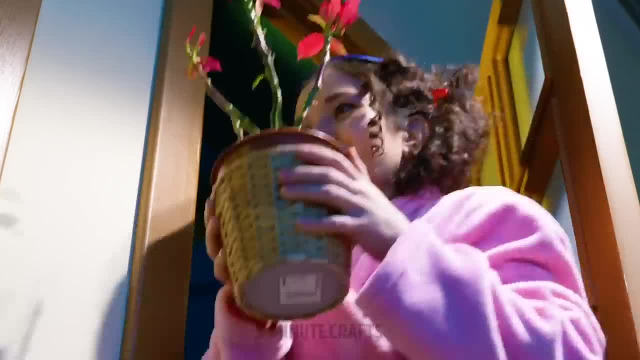 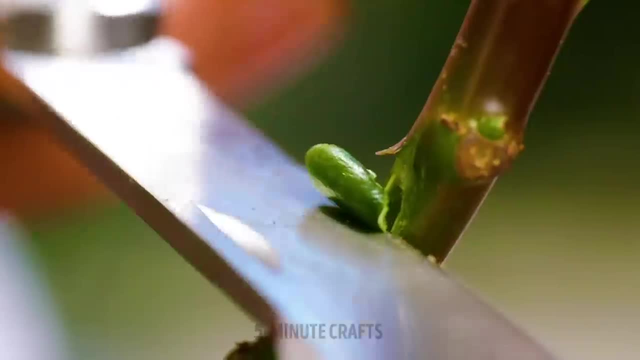 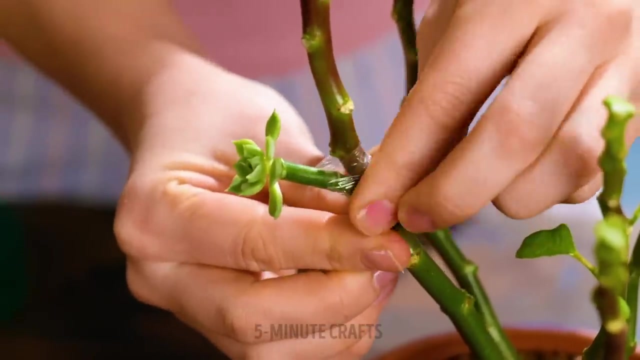 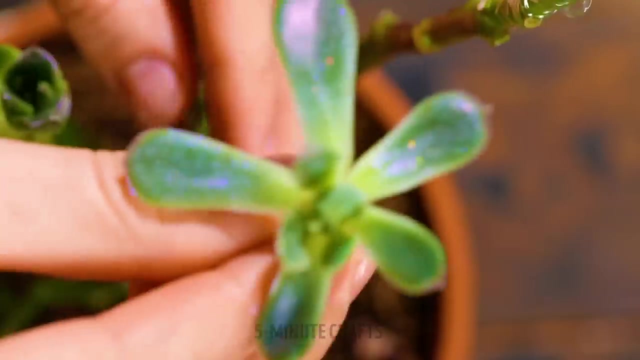 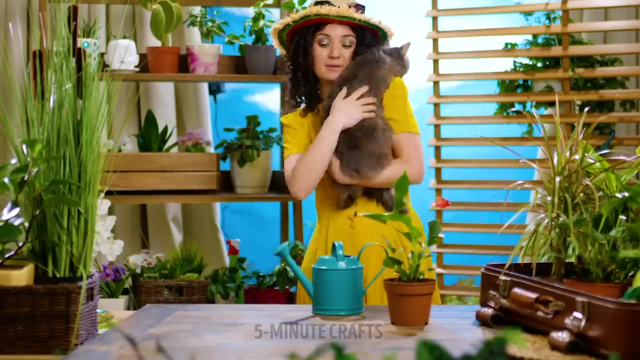 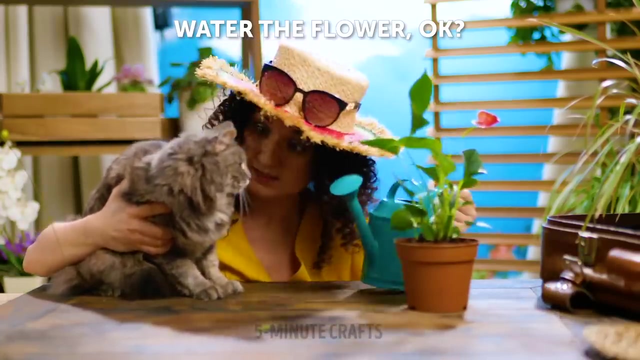 I've changed my ways, Cause I just want you back again And I know, hey, I am here to stay, There's no other way. So we don't fall apart. Don't keep your heart away. Try another day. So we don't fall apart. Let me stay here for a while. 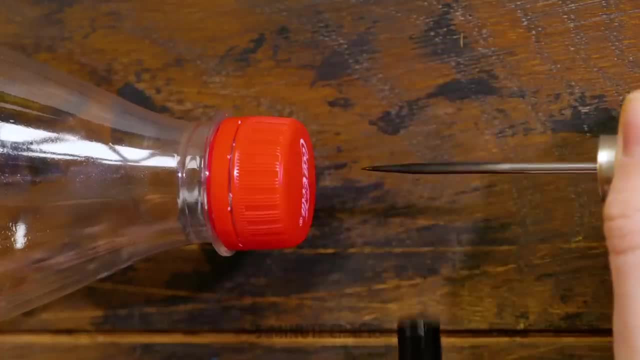 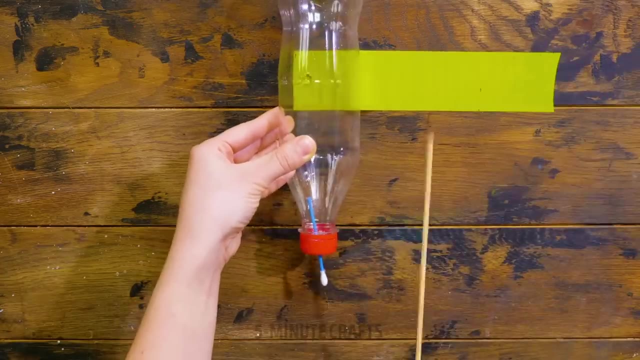 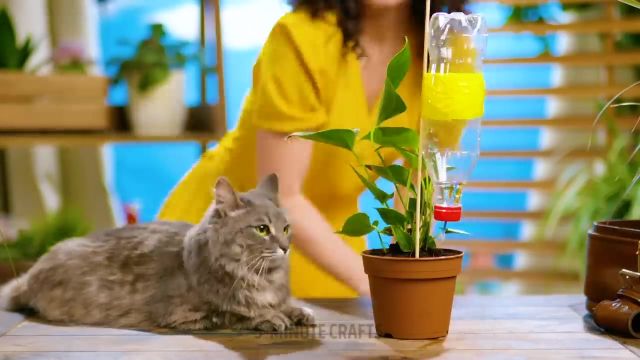 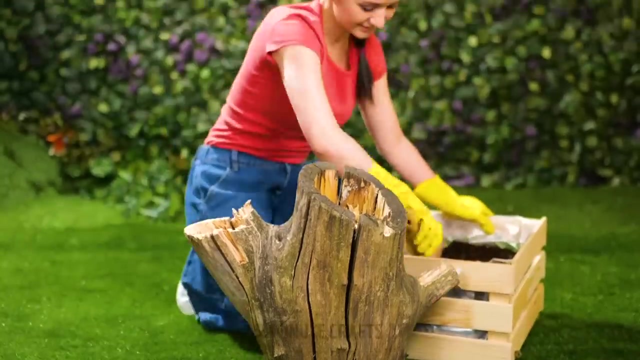 Look into my eyes for something right. Can we do this once again? You've already left town And I don't believe it, Baby. I don't believe it Tells my head: I am here to stay. There's no other way. So we don't fall apart. 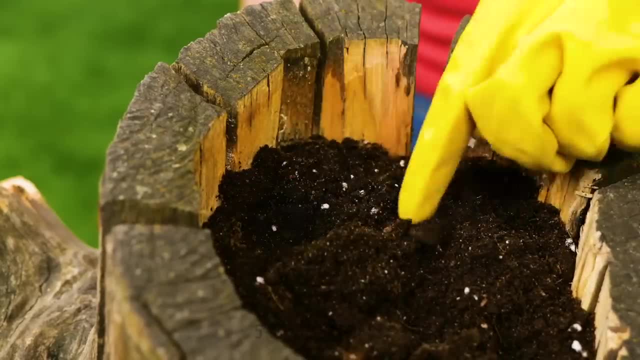 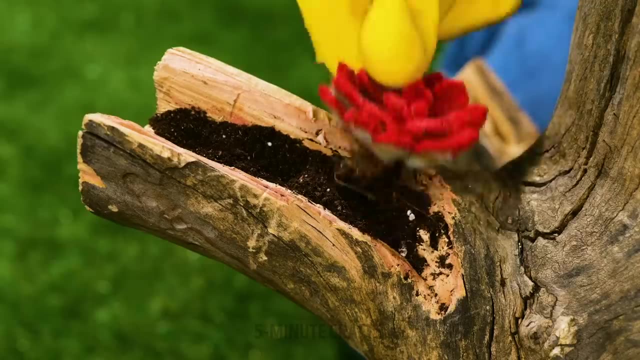 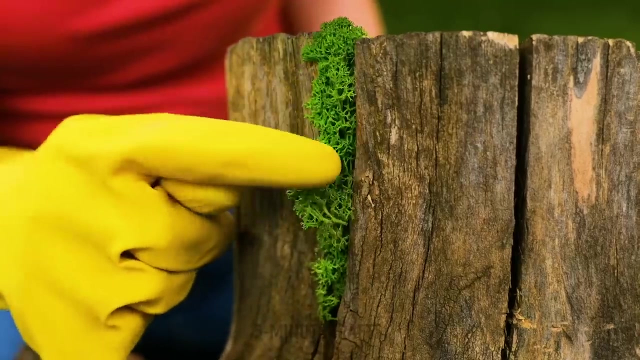 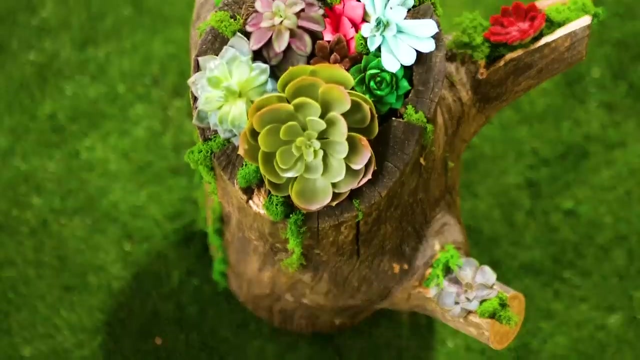 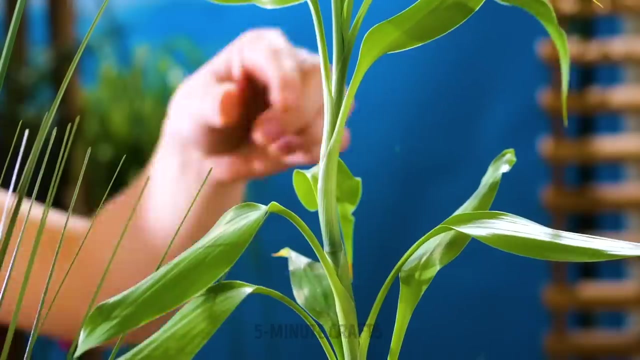 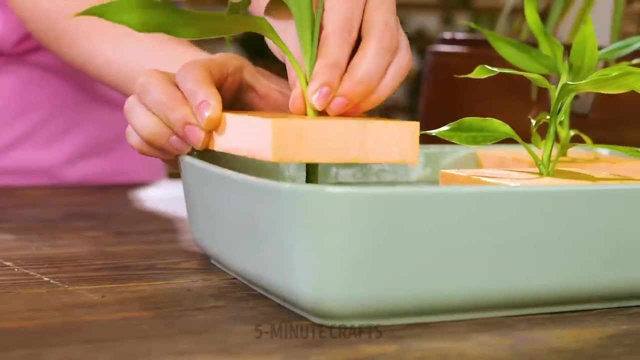 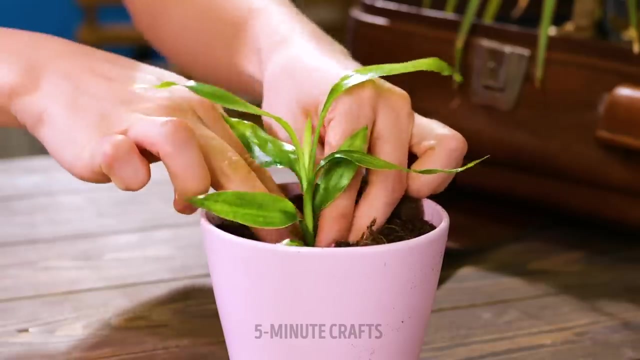 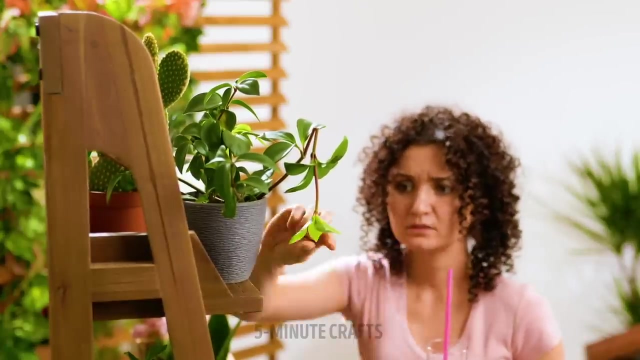 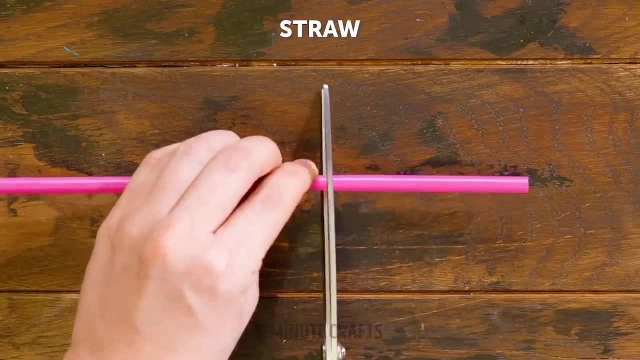 Don't give your heart away. Just try another day. So we don't fall apart, We start running. We're running From the world outside, Something's calling. If we lose it all, Can we keep ourselves from falling? And I know, hey, I am here to stay. 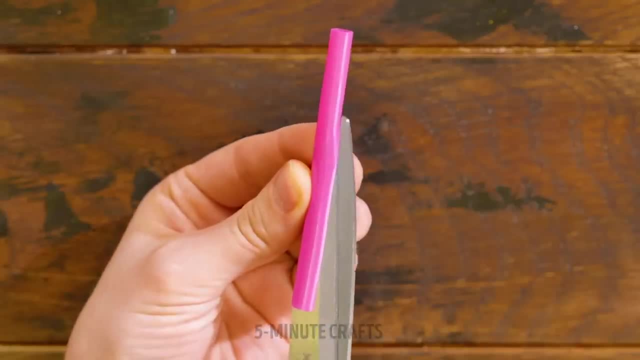 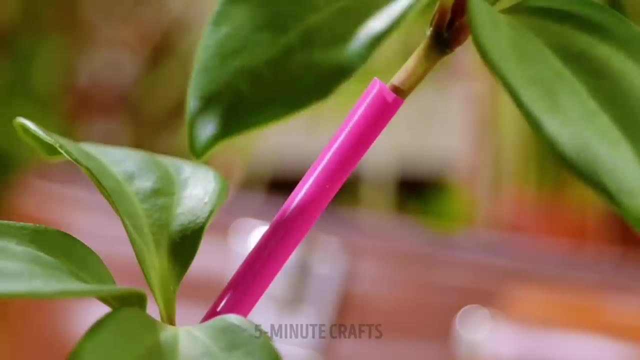 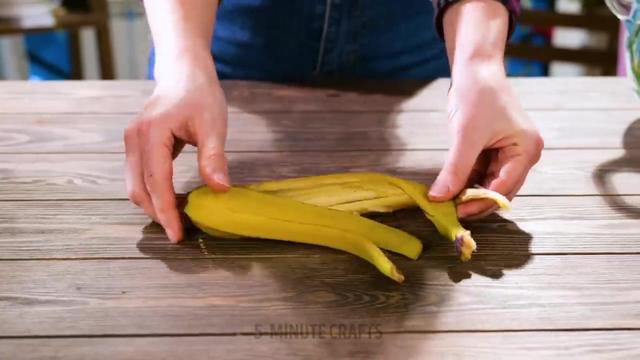 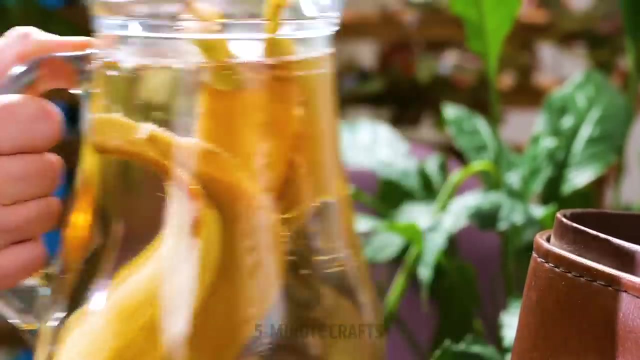 There's no other way. So we don't fall apart. Don't keep your heart away. Just try another day. So we don't fall apart, We start running. We start running And I know we have to. Yeah, We started acting like that And you never found what we had. 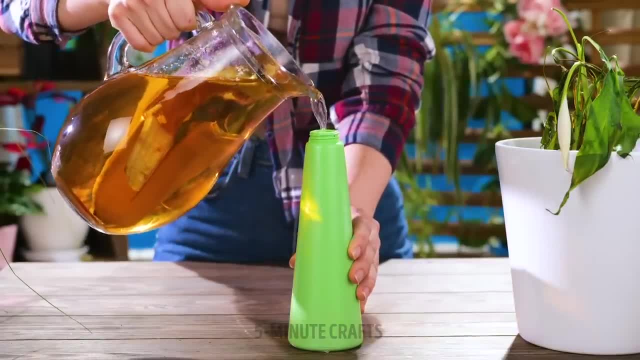 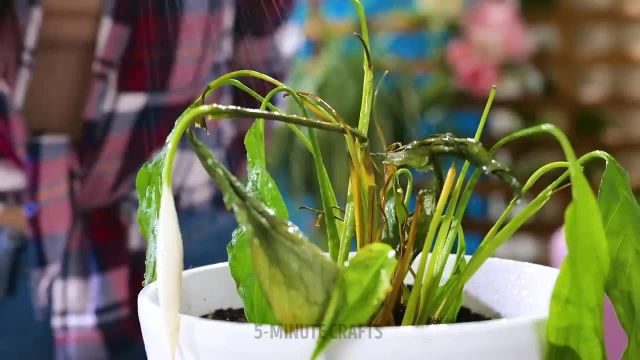 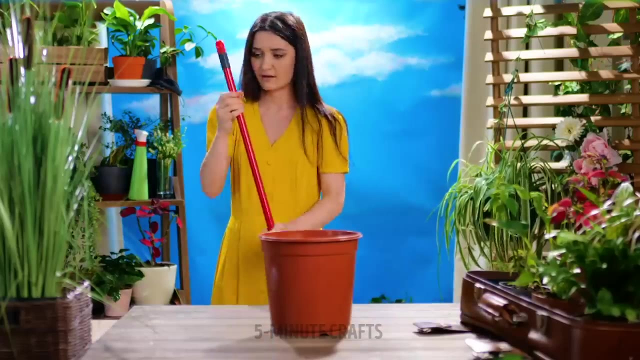 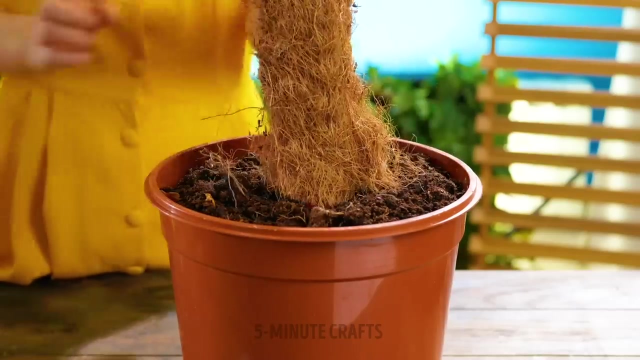 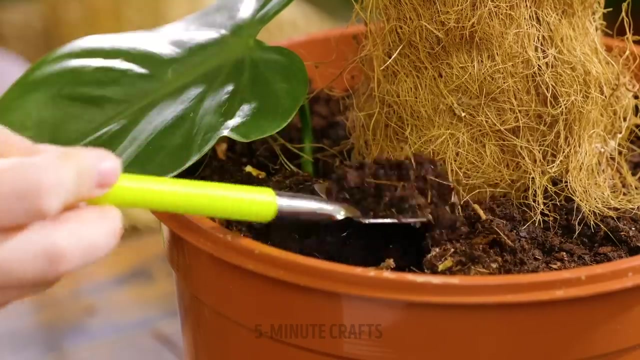 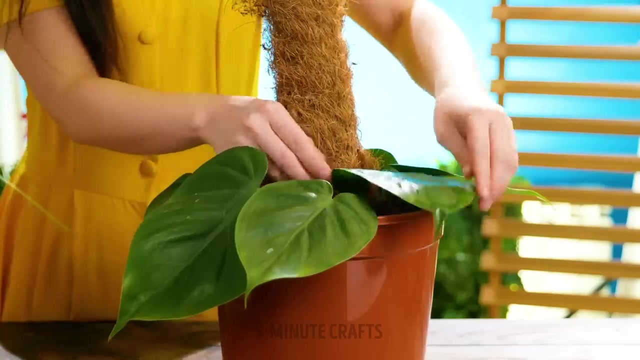 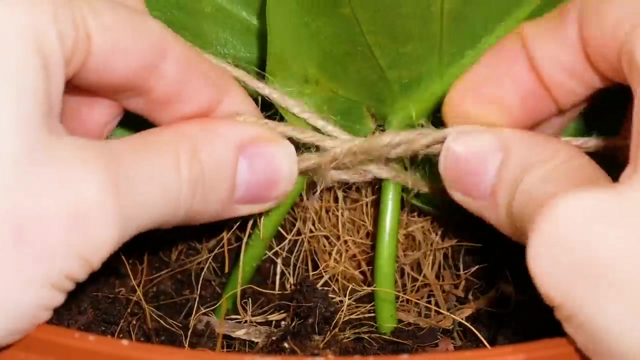 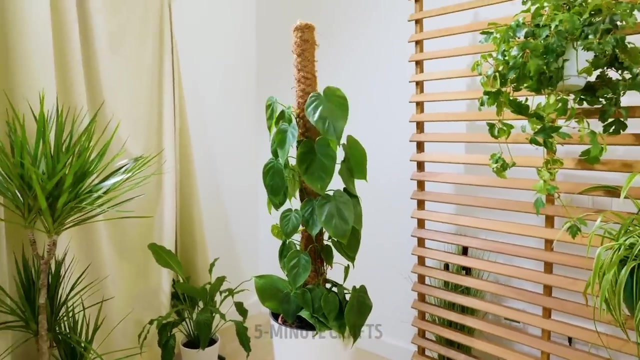 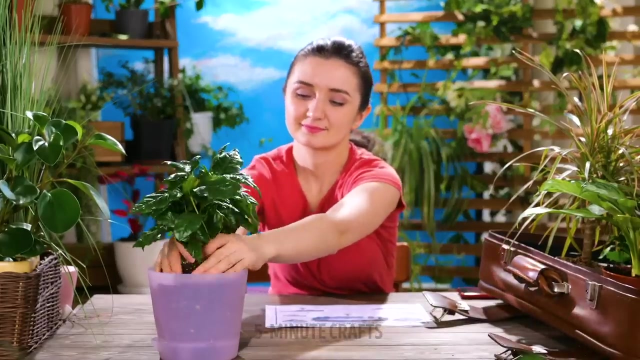 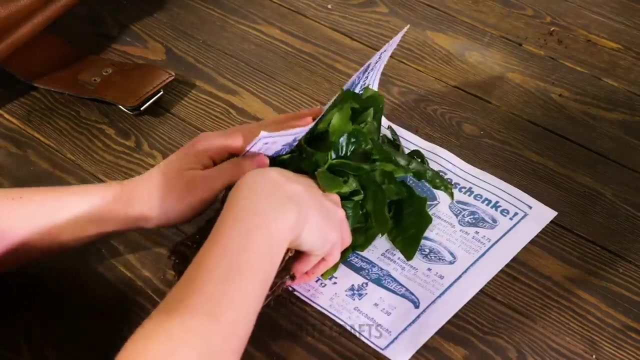 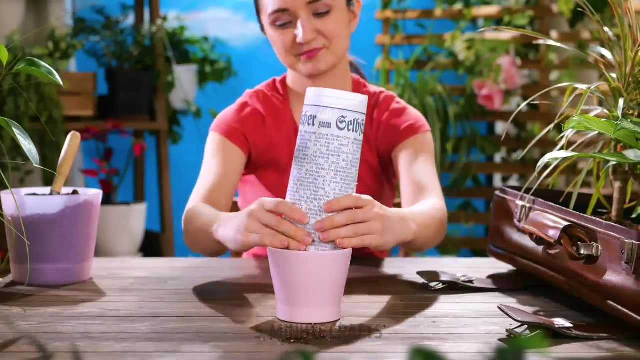 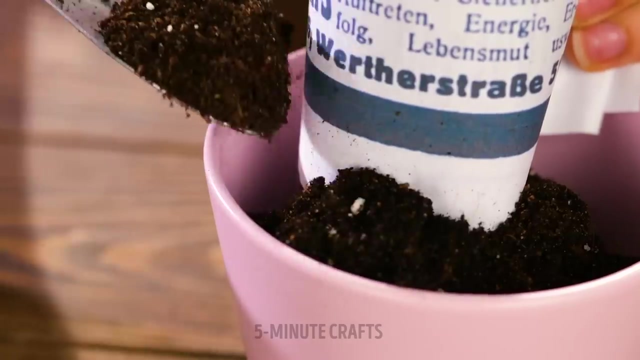 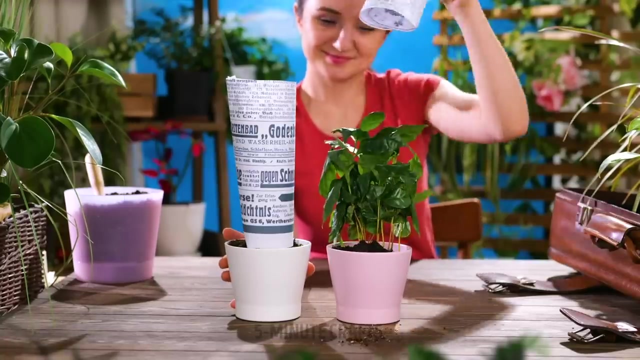 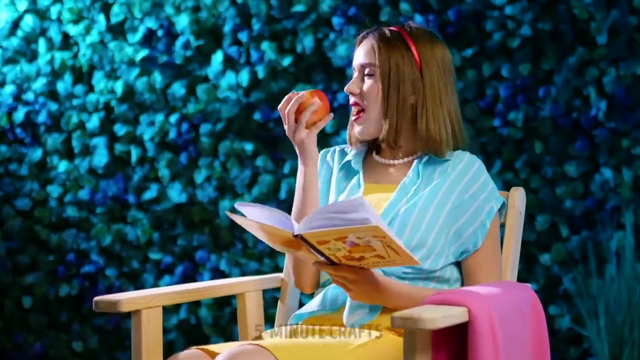 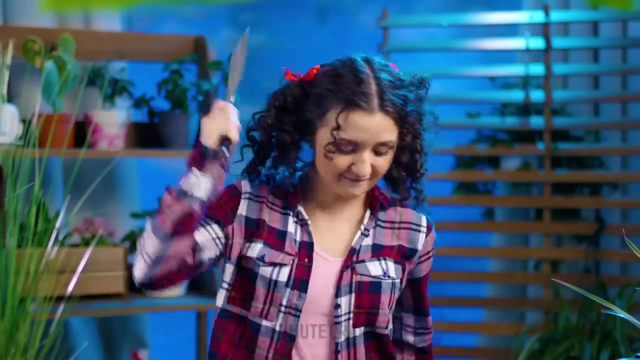 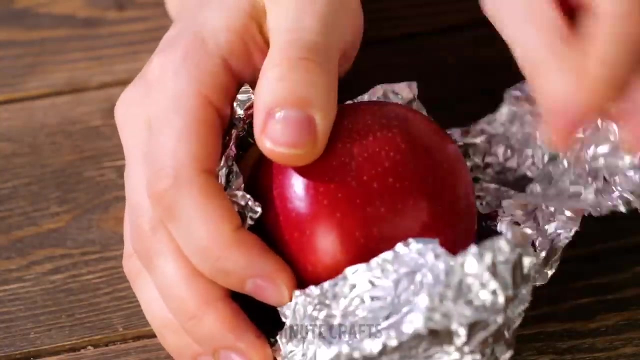 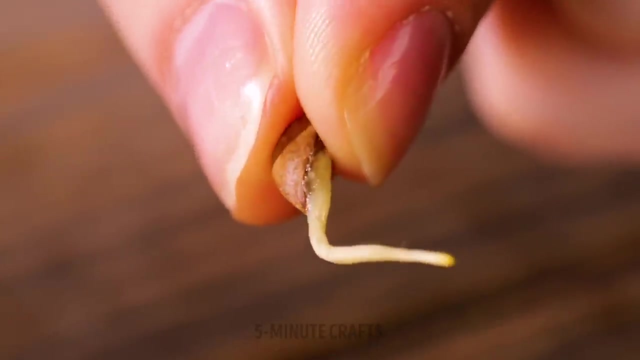 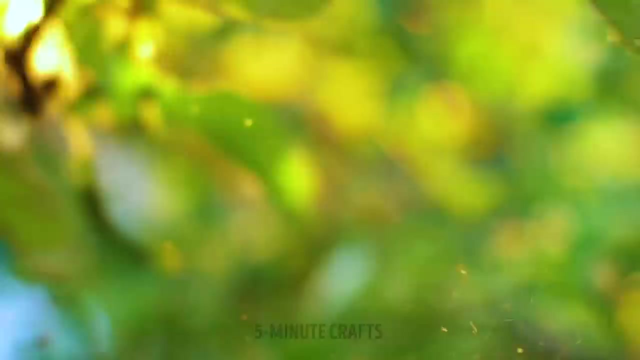 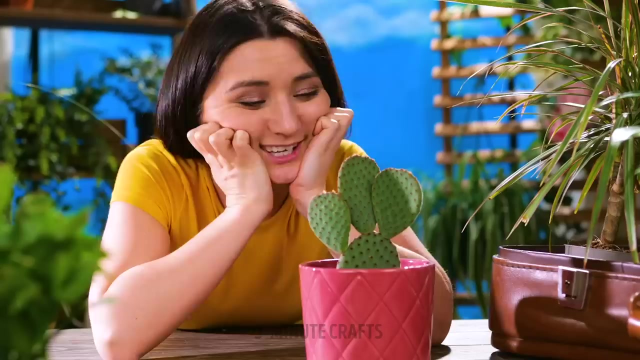 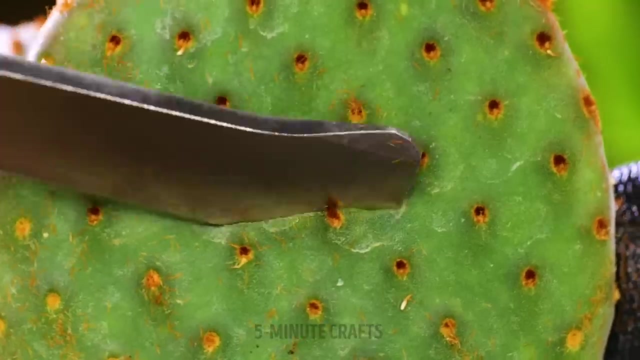 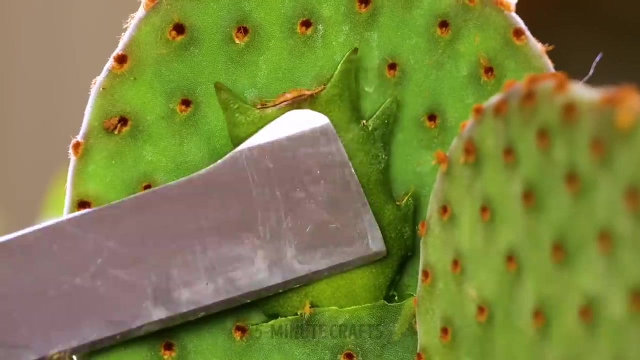 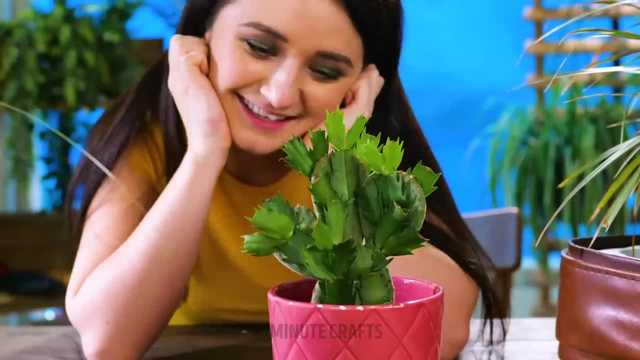 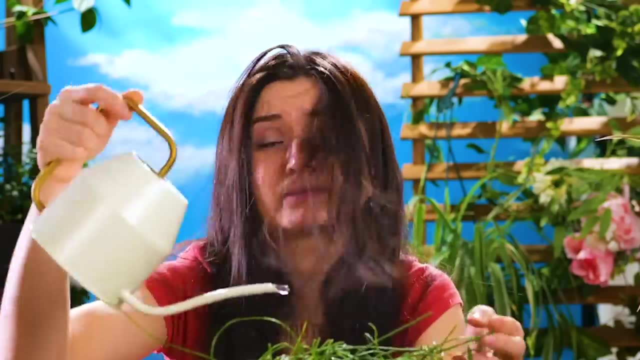 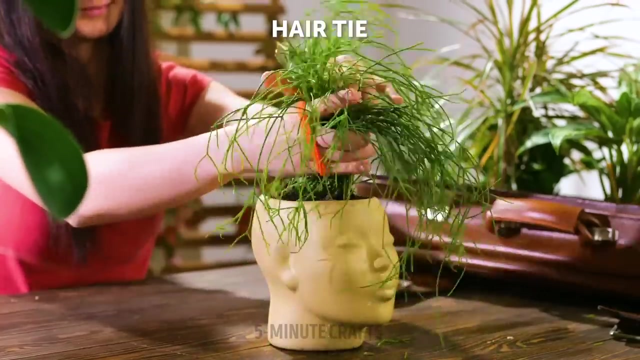 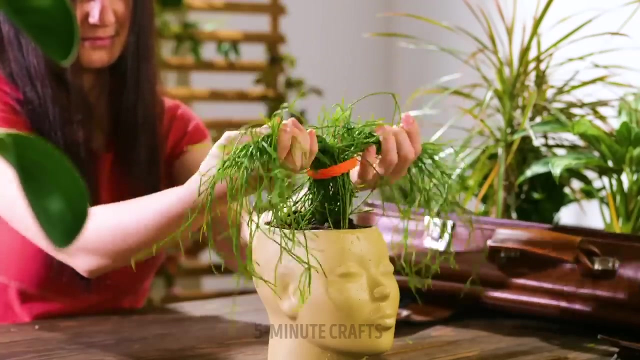 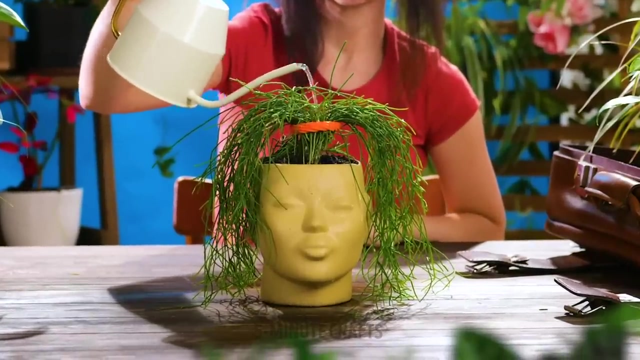 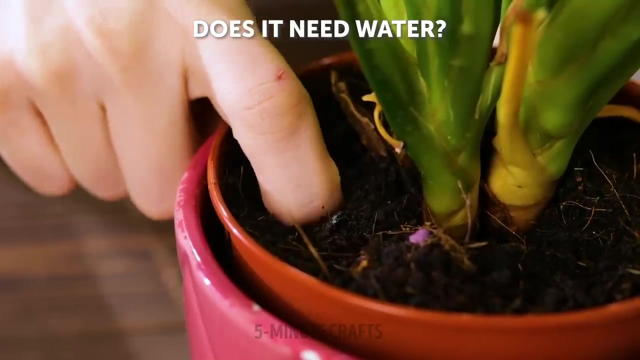 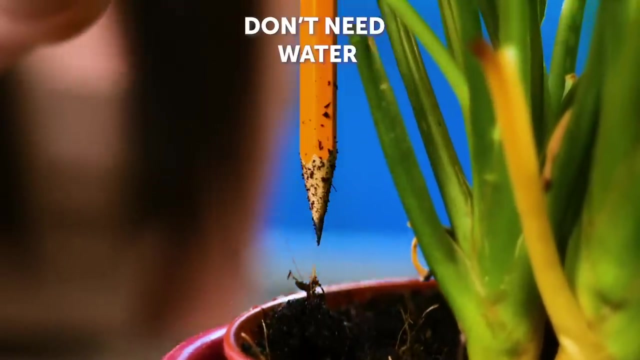 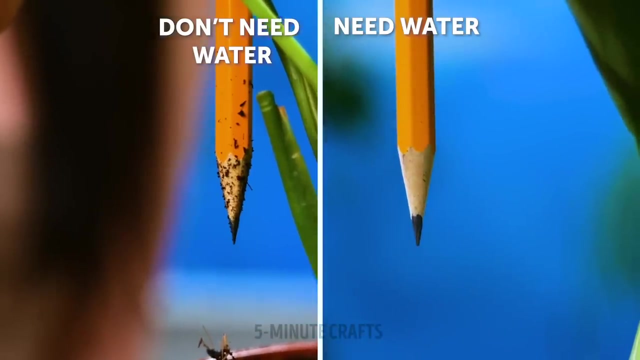 We'll be right back. We'll be right back.